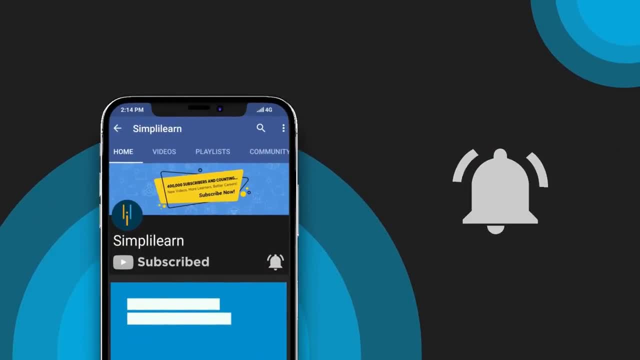 Hello everyone, welcome to yet another exciting video by simply love. Today we will go on a quest to uncover commonly asked logical reasoning questions in an aptitude test and the topics they are based on. We will go through all these details one by one, so stay tuned. 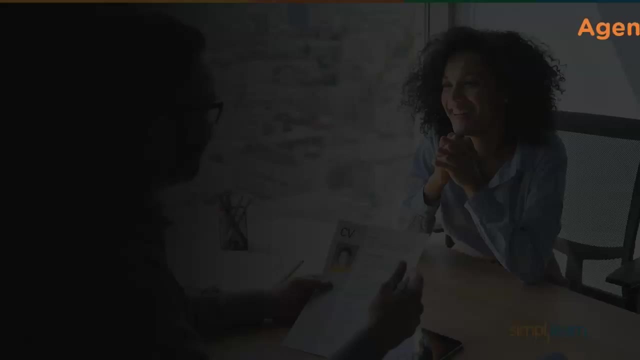 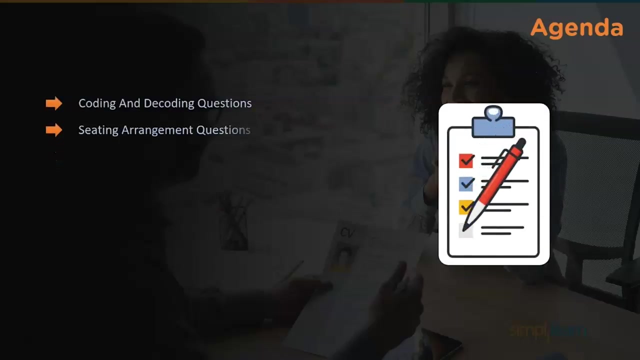 until the end of this video. At first we shall look into the agenda for today's session. The section that carries more weightage in logical reasoning tests are coding and decoding. sitting arrangement series, completion, direction, sense, blood relations, clock and calendar. 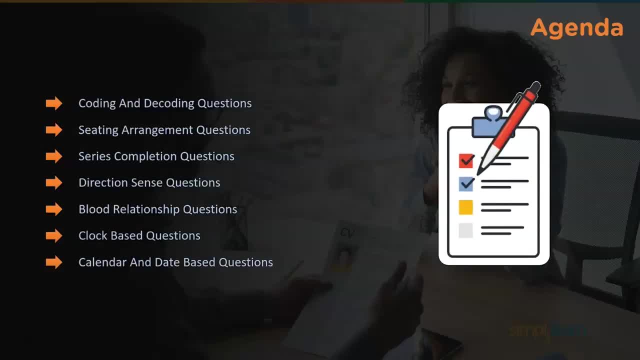 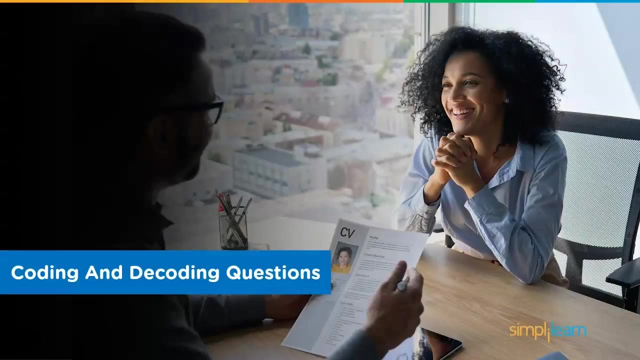 based questions. We will delve over details of all these categories one by one, But before we begin, make sure to subscribe to our channel and hit the bell icon to never miss an update. The first topic we are going to cover is coding and decoding. This section is one of the most 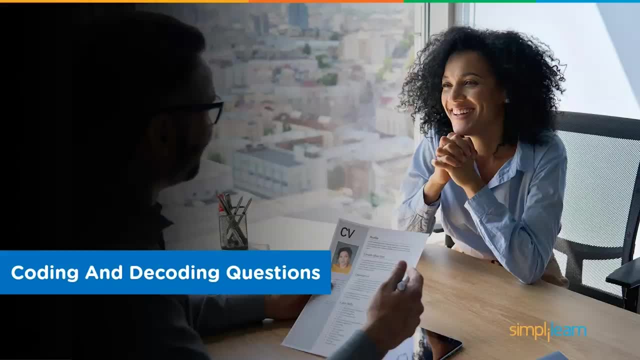 common sections included in all major exams conducted across the country. Many students find coding and decoding questions quite difficult. Thus they avoid attempting these scoring questions and thereby lose some easy and quick marks. We will look into the basics of these concepts to elevate our chances of tackling these questions. 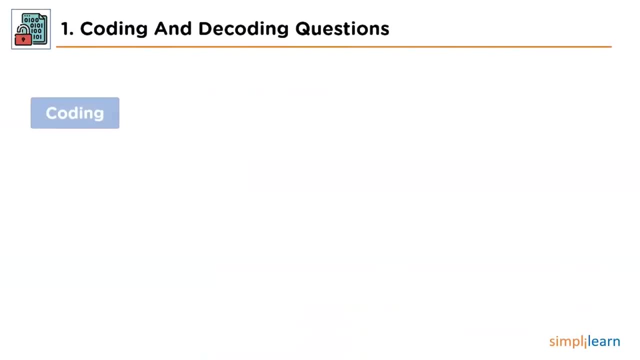 First let's understand coding. Coding is a part of the logical reasoning section used to encrypt words, numbers in specific patterns or codes using particular rules and regulations. In more technical terms, it is also referred to as encryption, and it is widely used across. 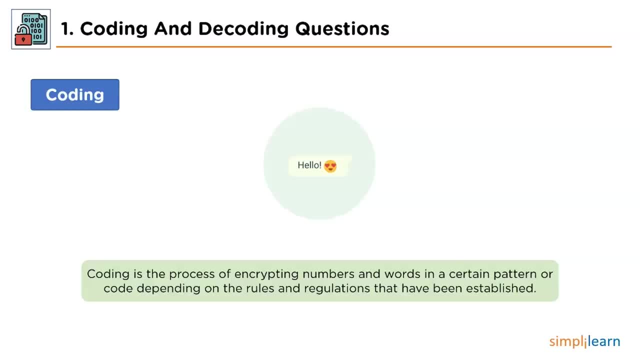 all messaging platforms to protect the contexts that users are communicating. The logic that these encryptions follow is known as key, which can cipher the context in no time. Let's have a look at an example to comprehend this better. The problem statement given here states that in a certain language, Kynomatophobia is written. 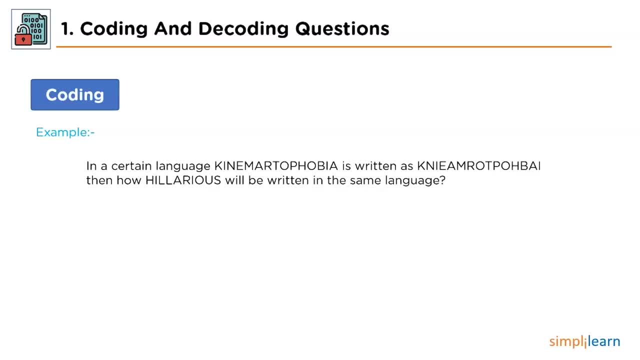 as K-N-I-E-A-M-R-O-T-P-O-H-B-A-I, Then, how hilarious. will be written in the same language. The logic to answer this question is engraved in the conversion of Kynomatophobia to KNIEAMROTPOHBAI. Let's take a closer look at an example to better understand this. First we can take a look at the same problem statement that was given in合 motivo. this time, The problem statement states that In a certain language Kynomatophobia is written. 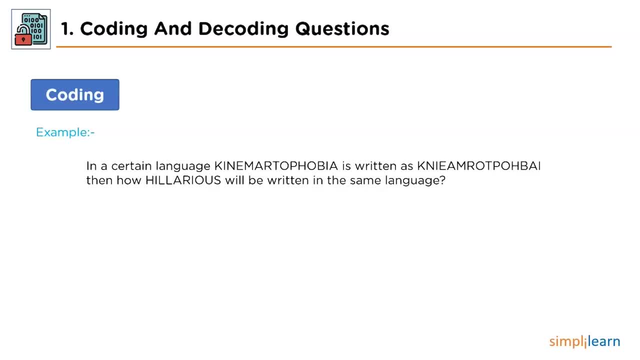 m-r-o-t-p-o-h-b-a-i. so let's take these words to our workspace and figure out the logic now. if you compare both these strings with one another, then you'll see that the logic of encryption is pretty clear. after every character, the next two characters are interchanging their 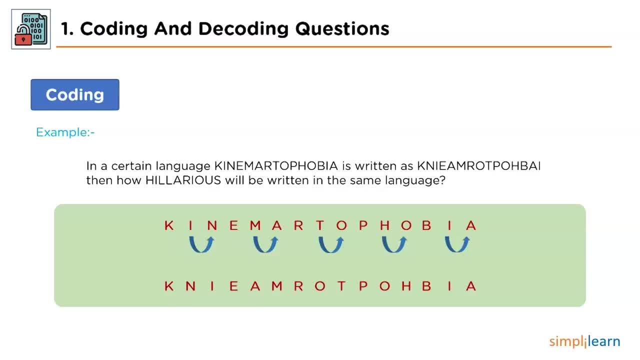 positions, as we have found the logic of coding here, so the next step will be to apply it to the question string. that is hilarious, so let's do that. the first letter will regain its position, and for the second position we'll have l and then i. after that, we'll keep l as it is, and 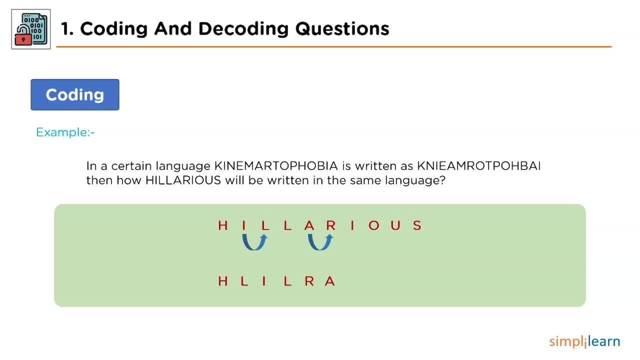 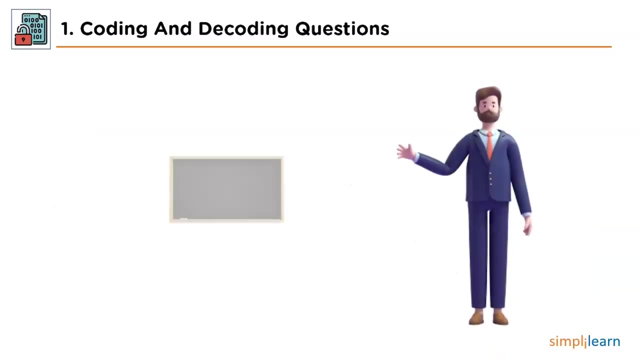 then we'll interchange position of a and r. next characters will be i, u, o and s. thus the answer to this question should be h, l, i, l, r, a, i, u, o s. on that note, here is a similar question for all of you, to gauge your understanding of the concept, the problem statement and. 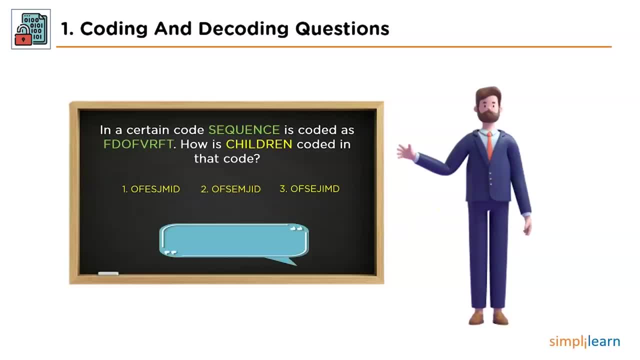 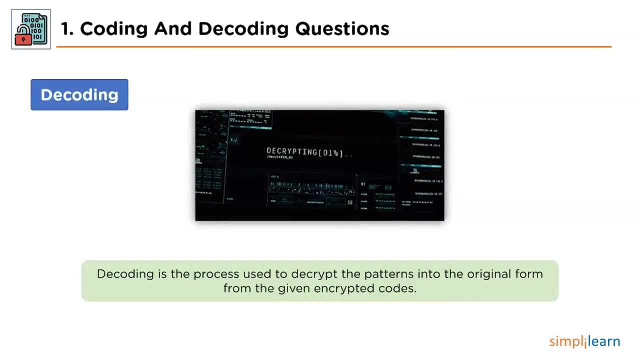 alternatives are given on your screens, so make sure to solve this problem and drop your answers in the comment box below. let's see how many of us can get this right. next we have is decoding. decoding is the process used to decrypt the patterns into original forms. in other words, to achieve decoding, you'll require the logic of encoding. 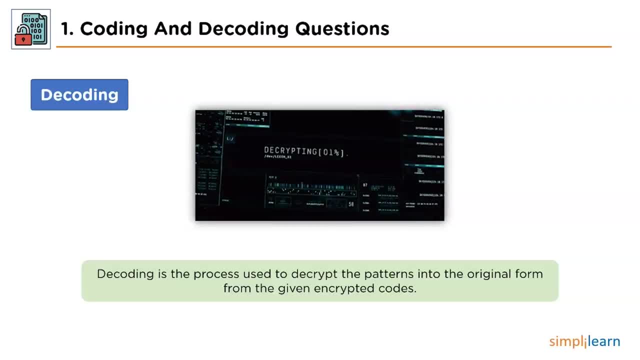 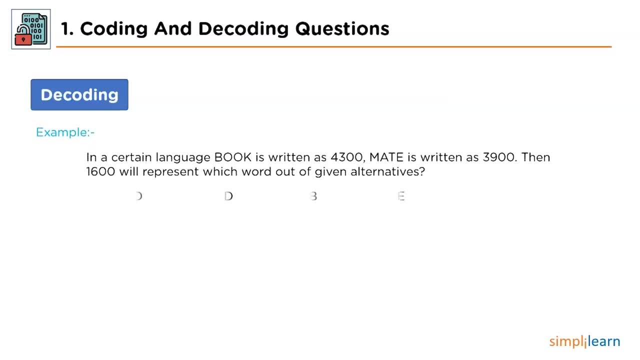 the first thing you'll have to do in this type of questions is to find the key of encryption or the logic behind encoding. let's look into the sample question to understand how these kind of problems work. the problem statement states that in a certain language, the word book is written as 4, 3, 0, 0 mate. 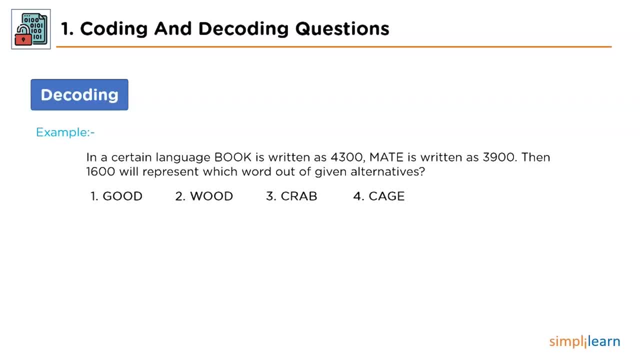 is written as 3 9 0 0, then 1 6 0 0 will represent which word out of the given alternatives? here we have been provided with two examples representing the logic of encoding, so let's look into each one of them one by one. 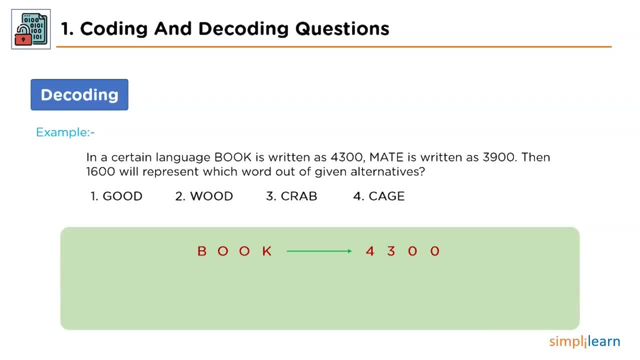 first we'll look at the encryption of word book. the word book has been converted into numerical format, so there must be some sort of relation between alphabetical numbering and number. 4, 3, 0, 0. so what we'll do is we'll take the reference from this. 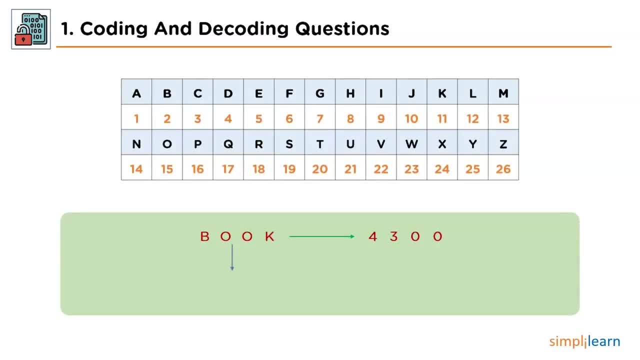 alphabetically ordered list. the characters b, o and k have position values to 15 and 11 and if you search the alphabetical numbering and numbering, you'll get the number 43. and if you sum all these values you'll get number 43. i don't think there is any logic behind those two trailing zeros. 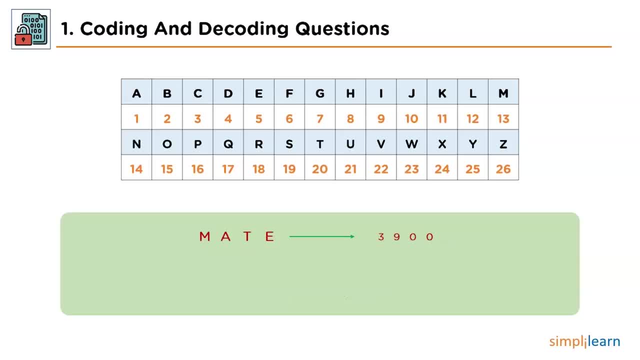 but we'll look into one more encoding example to ensure that the next string is mate, which is encrypted as 3900. in this case, character m, a, t, e have alphabetical positioning values 13, 1, 20 and 5 simultaneously, and the summation of these values will be: 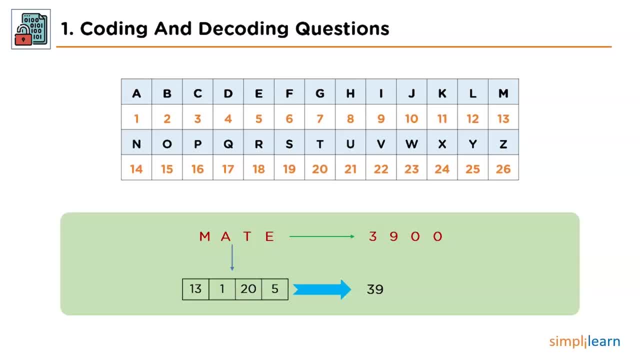 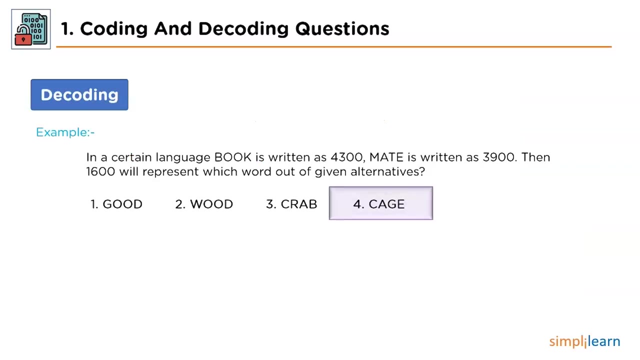 surely 16 and the corresponding value of 16 is the appropriate one, meaning the logic that we have found out is the appropriate one. from the previous two coding examples we can say that the right answer should have 16 as a character summation value and the only option that has 16 character summation value. 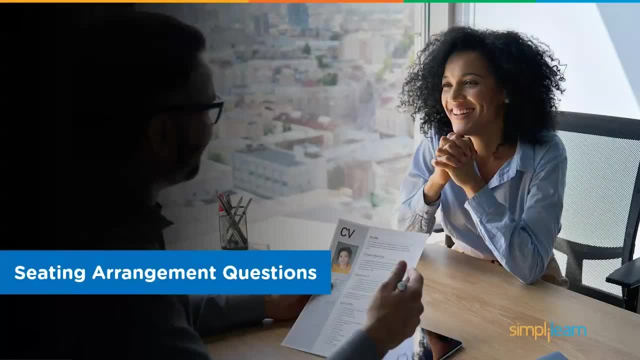 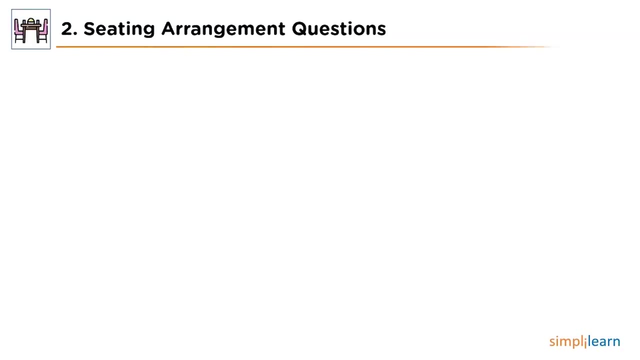 is gage, which is option 4 in this scenario. next we have is sitting arrangement. these questions We will have to understand the seating sequence direction- is the person facing inwards or outwards, etc. to be able to conclude the answer. These sorts of questions include straight line seating arrangement, complex seating. 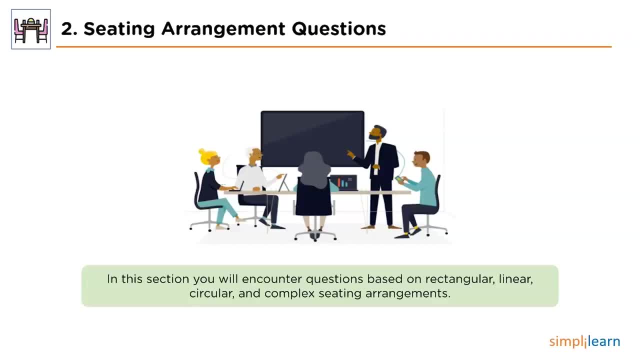 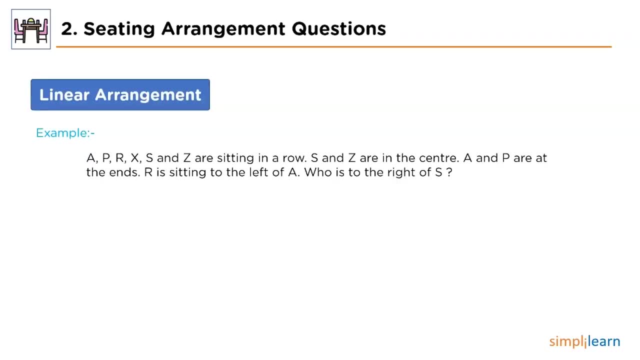 arrangement, such as circular, rectangular and triangular arrangements. First we will solve the sample problem based on the linear seating arrangement. The problem statement conveys that A, P, R, X, S and Z are sitting in a row. S and Z are. 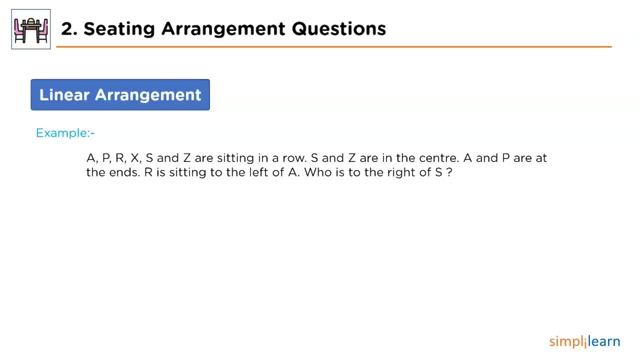 in the centre. A and P are at the edge. R is sitting to the left of A, then who is the right of S? From the first statement itself, we can say that we are supposed to arrange 6 persons in a straight line. 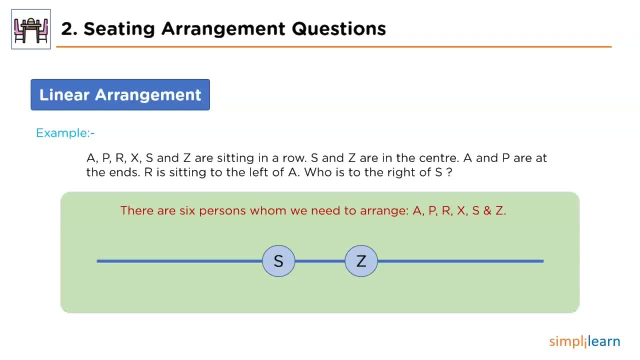 The next statement says that S and Z are sitting at the centre, so we will place them in the centre part of straight line Moving forward. the problem statement says that A and P are sitting at the end of our straight line, so we will arrange them as well. 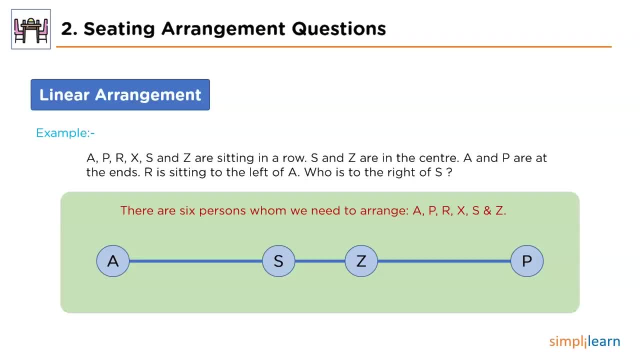 The next statement says that R is sitting to the left of A, but as there is no left position to the A, we will interchange position of A and P, And now certainly we can add person R to the left of A. Now there is only one position left, so we will place X over that position. 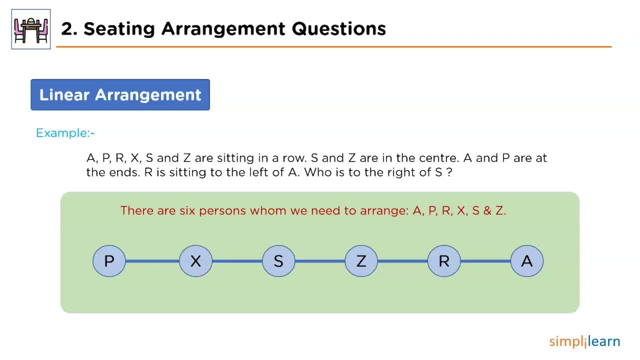 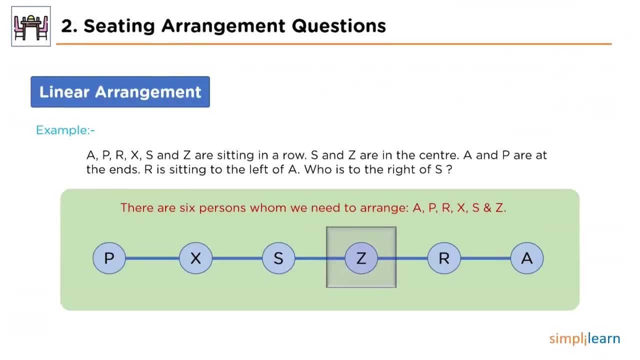 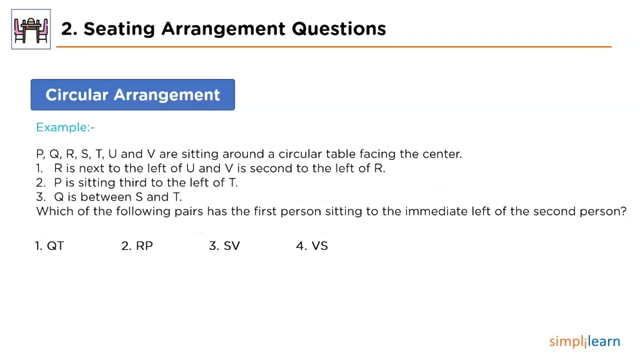 As all the persons are arranged in a straight line, we can draw an inference about who is sitting to the right of S, And the answer to this question is Z. Moving ahead, we will look at the sample question of circular sitting arrangement. The problem statement given here states that P, Q, R, S, T, U and V are sitting around. 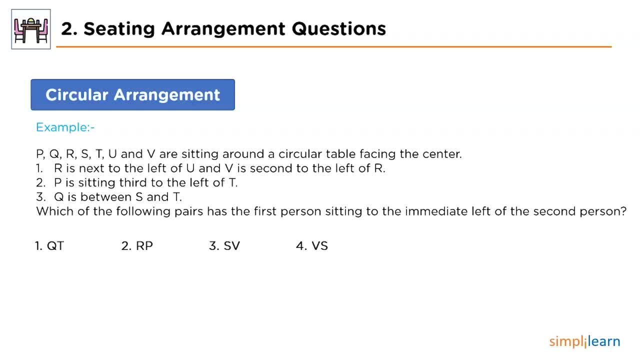 a circular table facing the centre, and there are 3 conditions that emphasize more about the positions around the circle. The first one is the position of the circle. The second one is the position of the circle. The third one is the position of the circle. 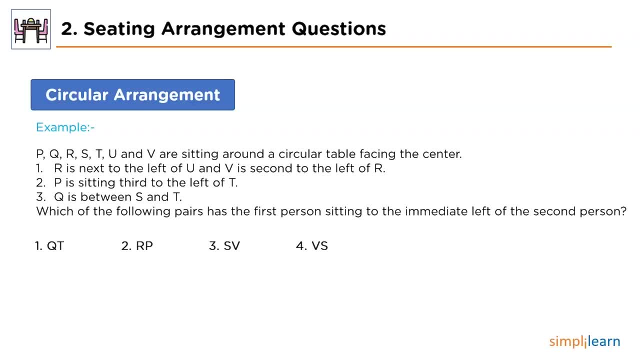 The fourth one is the position of the circle. The fifth one is the position of the circle. The sixth one is the position of the circle And the last condition says that R is next to the left of U and V is second to the left. 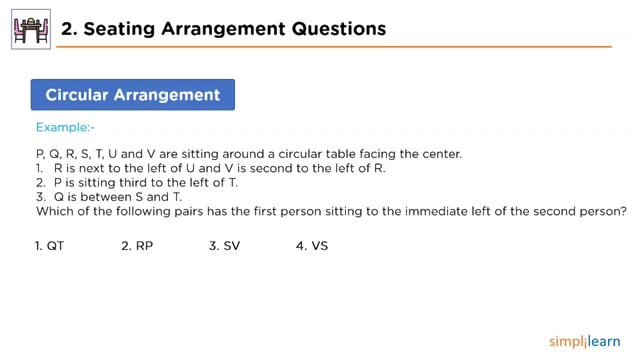 of R. The next condition entails that P is sitting third to the left of T and the last condition says that Q is between S and T. By using all these three conditions we are supposed to find out the alternative pair that has the first person sitting to the immediate left of the second person. 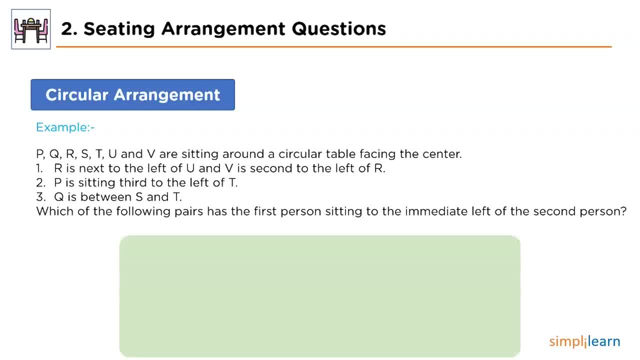 Let's formulate a solution to this problem. At first, we will add a circular shape and we will also say that also place 6th placeholder onto it, representing the 6 persons sitting in a circular pattern. Now, looking at first condition, we'll fix the position of R at any random placeholder. 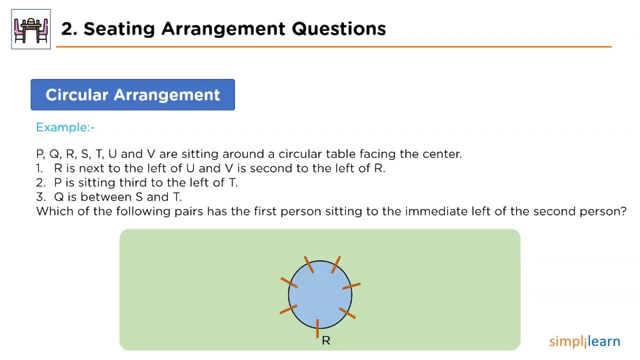 to figure out the position of other people. Reading the half part of first statement, that is, R is next to the left of U, you can draw an inference that U should be the right of R, So we'll assign the position to U as well. Moving ahead, let's deal with other half of. 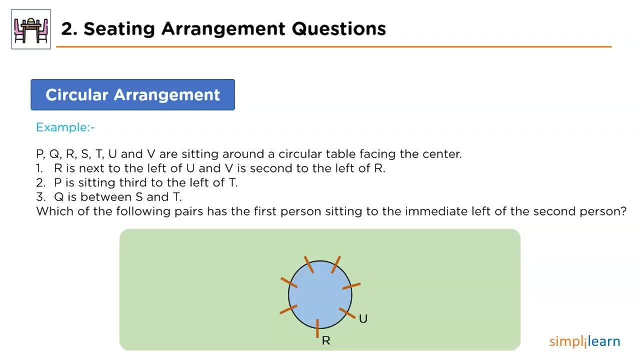 first statement. It says that V is second to the left of R. Thus, at the second left position of R we'll place V. Going to the second condition, which says that Q is between S and T, That means to place Q, S and T. we'll certainly need 3 empty positions close to. 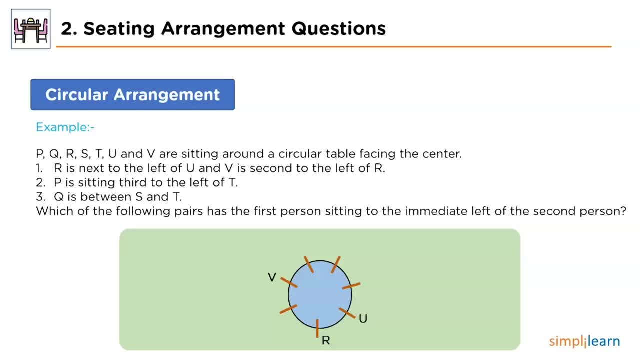 each other, and there is only one group with three empty positions, that is between V and U. Hence we'll add S, T and Q there. Also, the second condition of our list says that P is sitting to the third to the left of T. 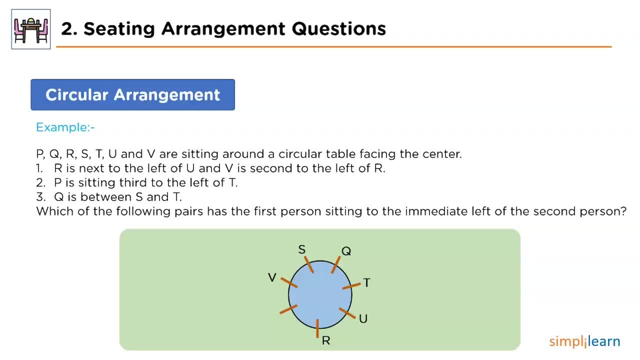 Now, by measuring the third left location from T, we'll add P to our circular arrangement. We have formulated the arrangement pattern, So let's dig up the right answer from all presented alternatives. The first option we have is Q, T. 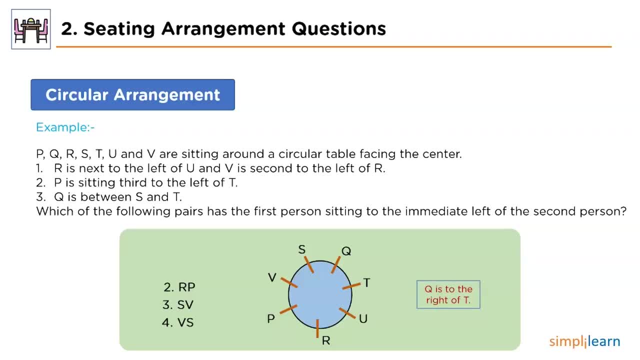 If you look at this option, you'll see that Q is sitting to the right of T, Hence we'll remove this option from our list. Then we have option R, P, And here also R is to the right of P. 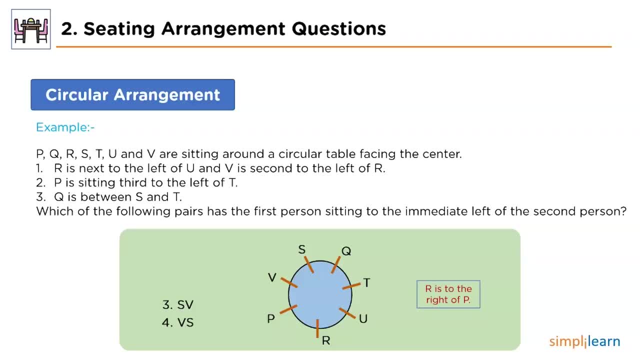 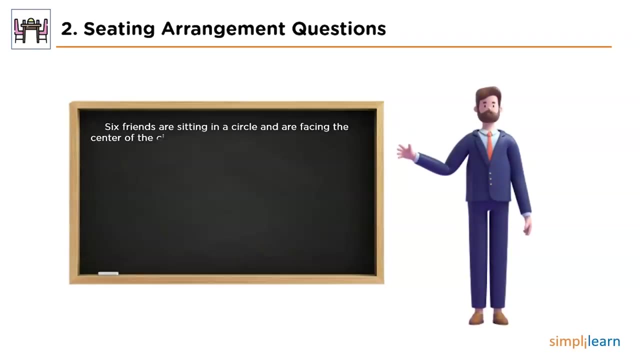 So we'll remove this option as well. Then we have S? V And S. S is available at the left position of V, Hence S? V is the right answer for our question. On that note, here is a similar question for all of you guys to gauge your understanding of sitting arrangement concept. 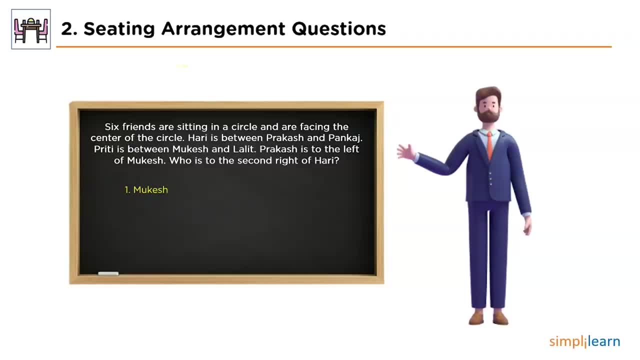 The problem statement and alternatives are given on your screens. So make sure to solve this problem and drop your answers in comment box below. Let's see how many of us can get this question right. Having said that, let's move to the next question. 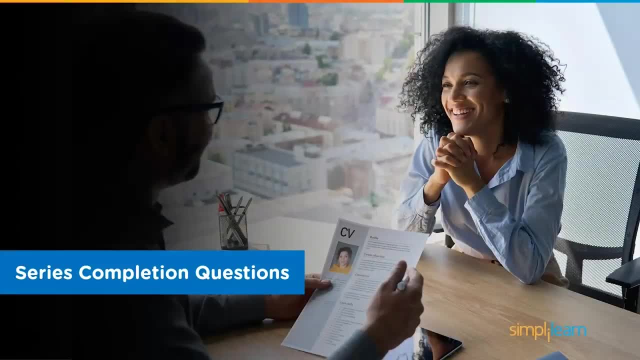 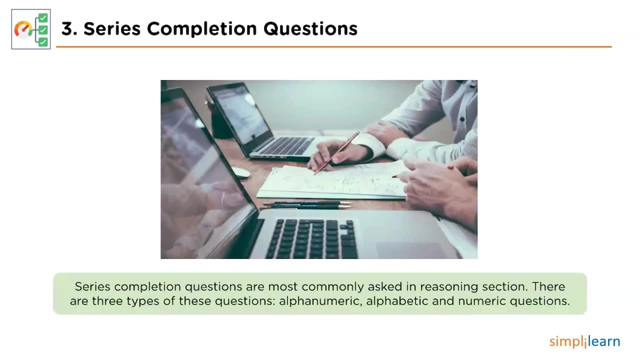 In this section the candidate is interested with recognising a pattern in a given set of numbers or letters. Then he'll have to pick up an option that follows the same pattern. Otherwise he'll have to identify the term that does not perfectly match the logic of given sequence. 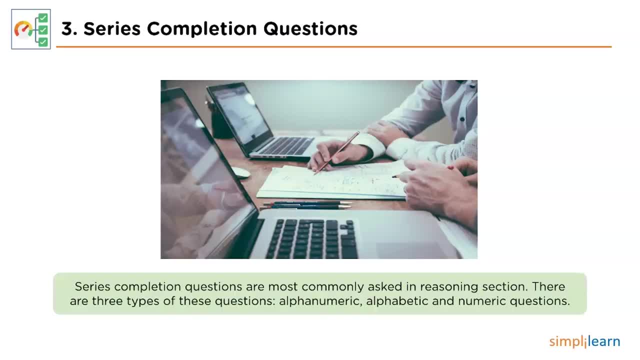 There are three types of sequences you'll come across in this series completion questions. First one is alphanumeric, Second one is alphabetic And third one is numeric. The main task you'll have to carry out is identifying the logic engraved in this set of numbers or characters. 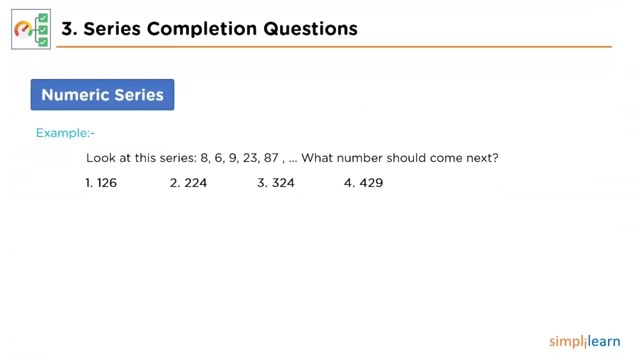 Let's look into the sample problem of series completion. The first problem of series completion is based on numerical sequencing, And the sequence that we have been provided with is 8,, 6,, 9,, 23 and 87. Let's take these numbers on our workspace to formulate an answer. 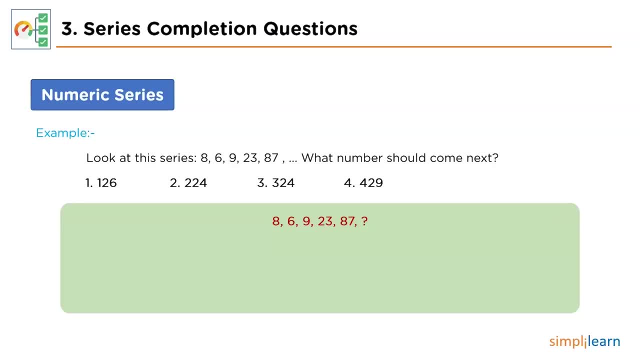 Now, if you observe these terms, you won't find any direct pattern, So let's break these numbers. We can derive the second term from the first one by subtracting 2 from it, But this pattern won't make sense for upcoming terms. 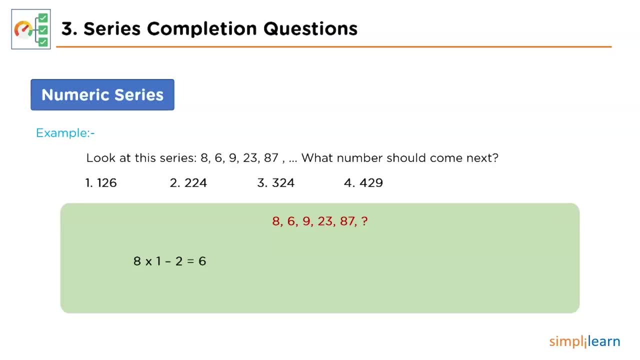 So what if we represent it as 8 multiplied by 1 minus 2.. Now let's try to relate this pattern to our next term. Here, if we represent it as 6 into 2 minus 3, then we'll get third number of our sequence. 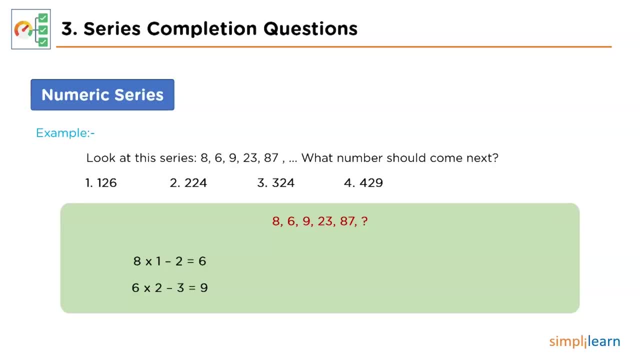 This suggests that we are in control of our sequence, So we'll be decreasing each break down by 1.. Let's take 9 now. 9 into 3 minus 4 is 23.. And similarly, 23 into 4 minus 5 is 87.. 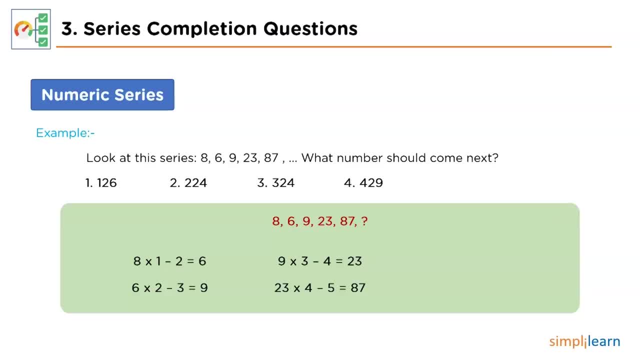 This means the pattern that we have found is correctly appropriate. Therefore, the next term will be 87 into 5 minus 6, which is nothing but 429.. Let's look into one more problem for series completion. This time the type of sequence we have is alphabetic. 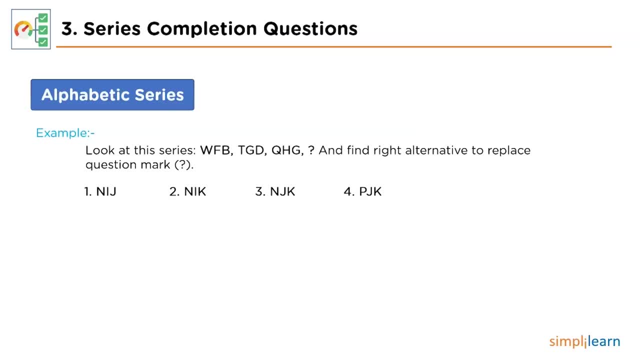 Which goes like W, F, B, T, G, D, Q, H, G and question mark. Here we are supposed to find out the alternative that can replace the question mark sign. So let's bring this sequence into our workspace to figure out an answer. 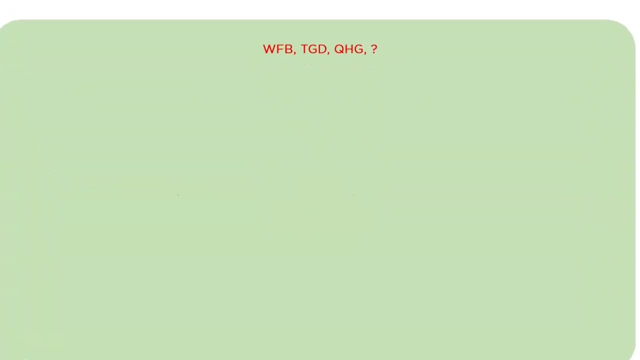 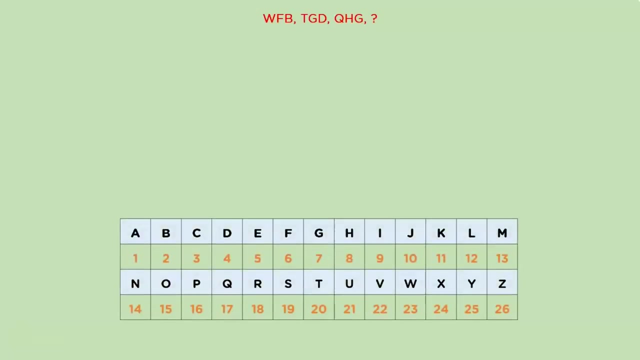 The logic for alphabetic sequence is most frequently embedded in the numerical ordering. Hence let's bring an alphabetic numeric table to consider their orders. Now, using the table values, we'll figure out consecutive sequencing for each character in all three terms. 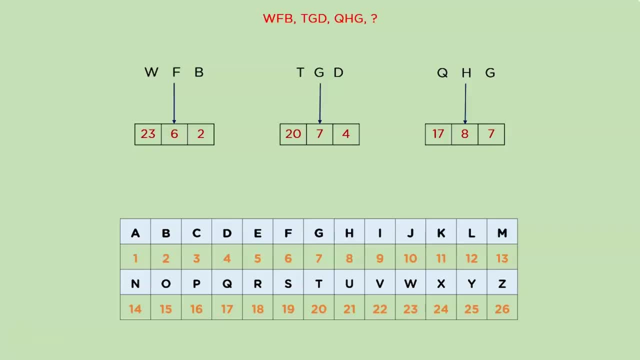 Now, if you look closely at each first character numbering for all three terms, you'll see the pattern: 23 minus 3 is 20.. 20 minus 3 is 17.. And 17 minus 3 should be the next character. 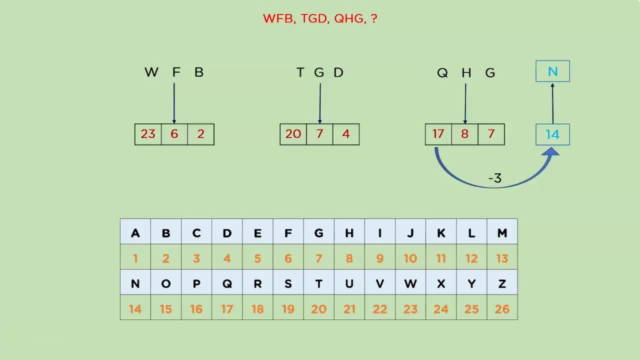 that is, with sequence number 14.. And that should be the character n. Now let's figure out the middle character of our next term. Here, if you observe, G is one place forward to that of F. Similarly, in third term, we have H, which is again one place larger than G. 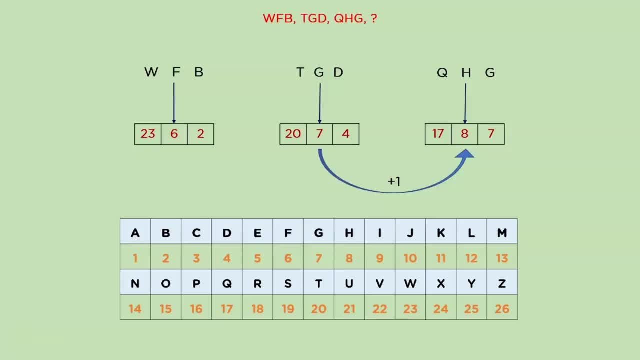 And by abiding by this logic, the middle term for our next term should be one place greater than H, which is nothing but I. Finally, let's discover the final character for our next term Here. if you observe, each character increases linearly with the value 1.. 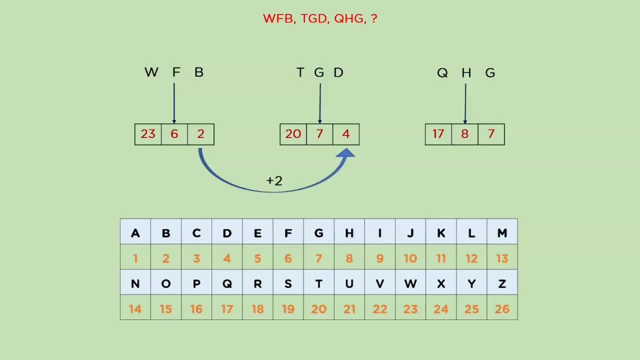 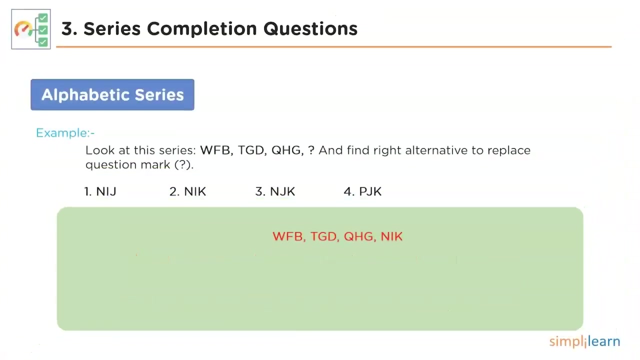 Hence the final character should be four places greater than G, which is K in this case. Now, by compiling all these characters that we have figured out, we'll get the right answer to our question, which is option B, NIK. 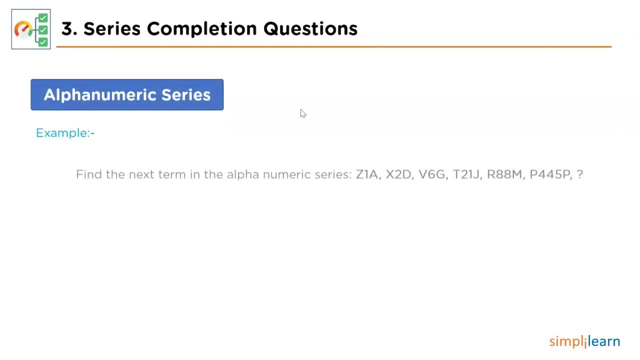 Moving forward, we'll look into the alphanumeric series problem. The sequence given here starts like Z1A, X2D, V6G, T21J, R88M and P445P, So we'll take this sequence on our workspace to figure out what this series is all about. 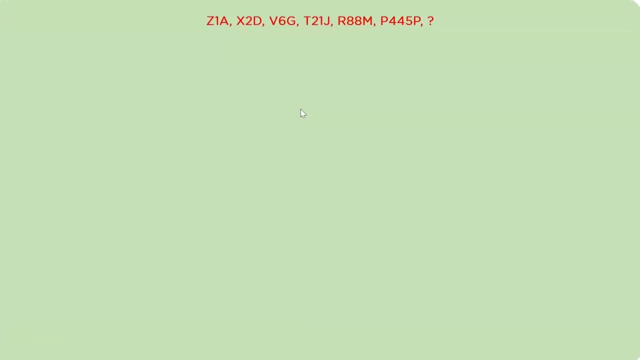 We'll break each term into three parts and we'll arrange it in tabular format. Let's first figure out the logic behind starting characters. If you observe this set of characters, you'll see that each step, one character has been omitted. 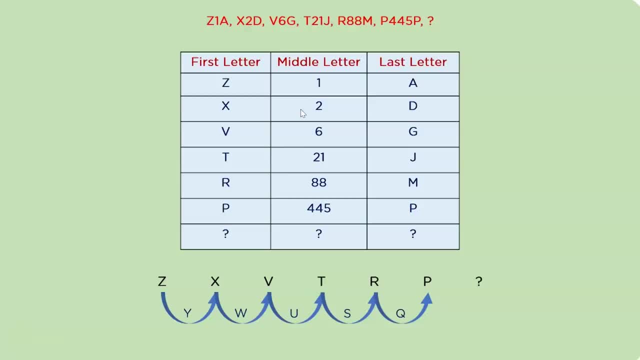 We have Z and X in this set, where Y has been omitted. Similarly, we have V and T, and the middle character out of them, that is, U, has been omitted, And if we apply the same logic, the next character should be N. 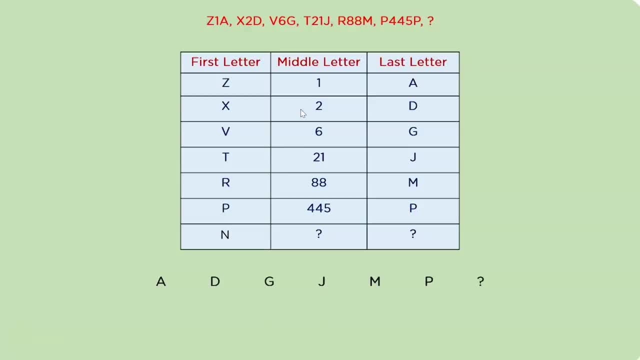 Let's figure out the last letter. In this case, two characters have been omitted for each inclusion. After A, we have D and after D we have G, which means we have omitted BC and ES. In accordance with the same logic, we'll discard the character Q and R and we'll include character S into our table. 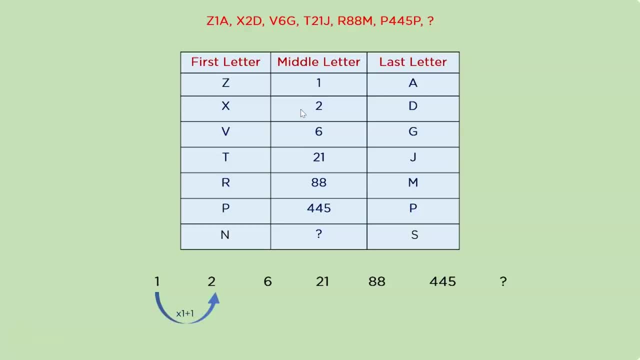 Finally, let's discover the middle part of our next term. Here each term is multiplied and added to the previous term with the increment of 1.. For example, the second term equals to the previous term into 1 plus 1.. The third term is equal to the second term into 2 plus 2, which is 6.. 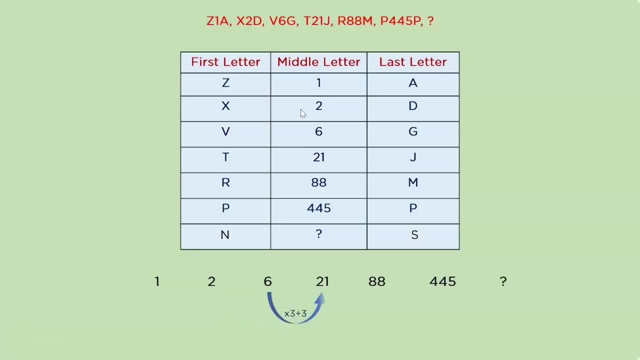 Next term is the third term into 3 plus 3,, which is 18 plus 3,, which is 21.. Similarly, the following term should be 21 into 4 plus 4,, which equals 88.. By following the same sequence logic, we can say that the next term should be 445 into 6 plus 6,, which is nothing but 2676.. 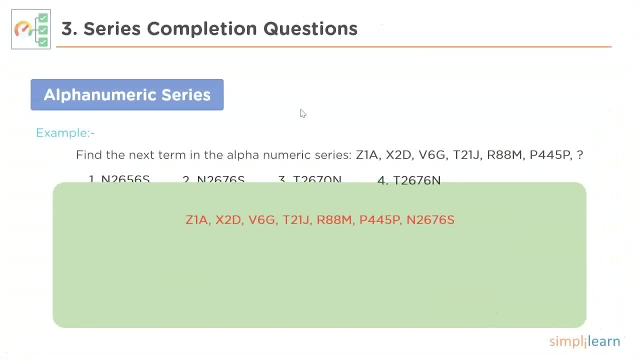 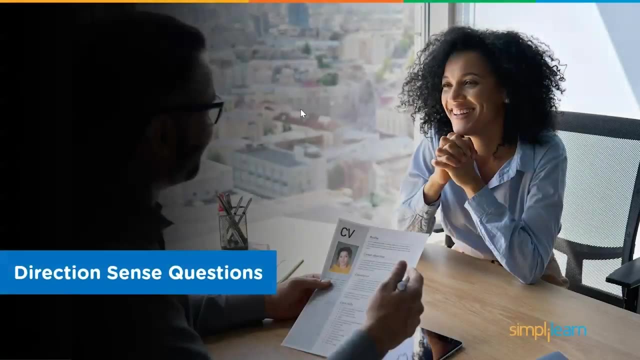 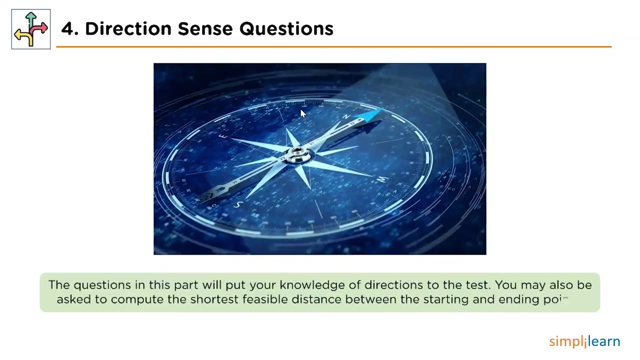 That means our answer is option 2.. Following this, we have direction sense. There are four main directions: east, west, north and south. Also, there are four cardinal directions, such as north-east, north-west, south-east and south-west. 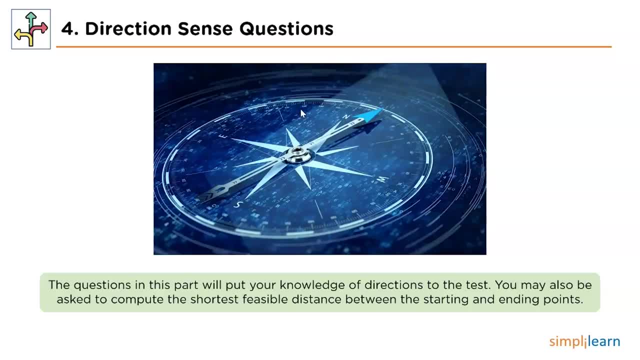 The questions in this section will test your understanding of these directions. You may also be asked to compute the shortest feasible distance between the starting and ending points. We'll look at one sample question to get an idea about the question. The problem statement given here states that 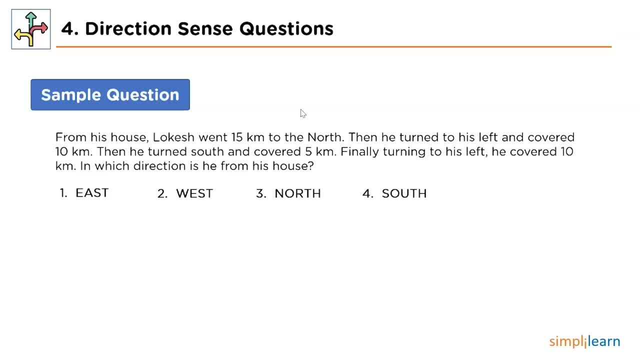 From his house. Lukash went 15 km to the north. Then he turned to his left and covered 10 km. Then he turned to south and covered 5 km. Finally, turning to his left, he covered 10 km. In which direction is he from his house? 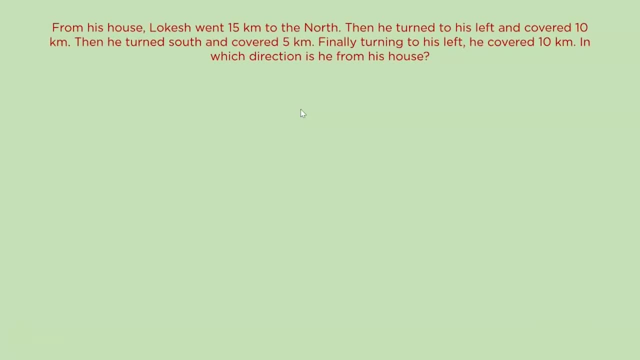 Let's figure out an answer to this question by tracing each statement. First of all, we will add a direction plot to make sure we get the answer plot right. The first statement states that Lukash went to 15 km north. This also means that we'll add a line in upward direction, marking it with a distance of 15 km. 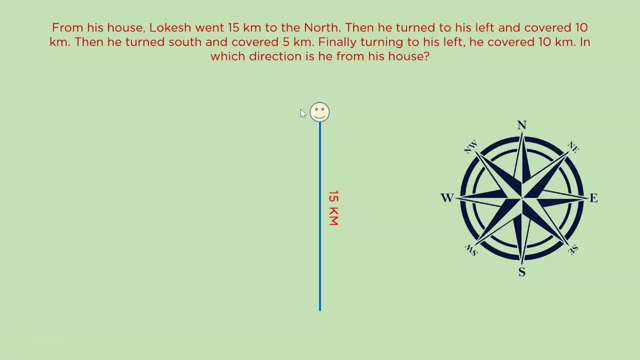 The next statement says that After covering 15 km towards north, he turned to his left and covered extra 10 km. His left side is west, so we'll add a straight line in that direction. The third statement conveys that Lukash turned to the south and walked 5 km. 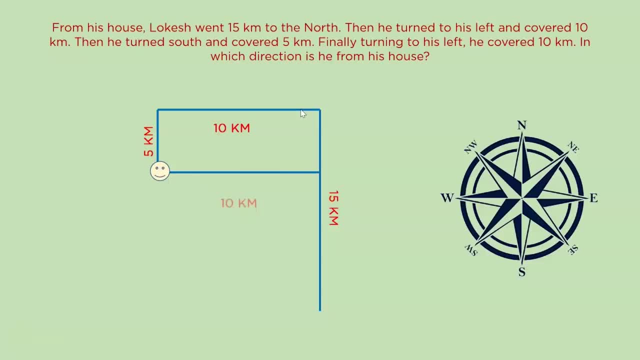 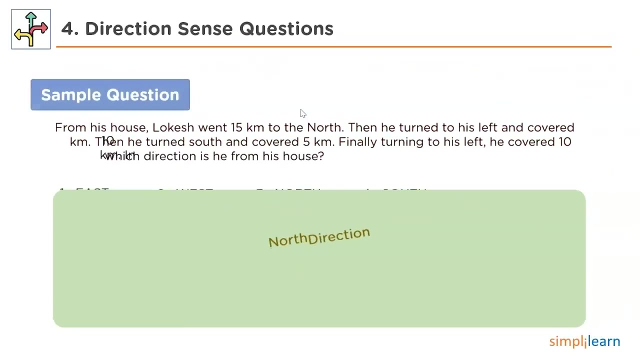 And further. he turned to his left and covered 10 km more. Now, if you trace his current location from the starting point that is his home, you'll see that it is in north direction. So the right alternative for our question is option 3.. 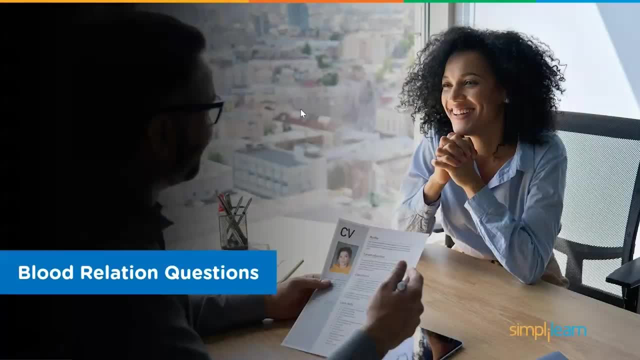 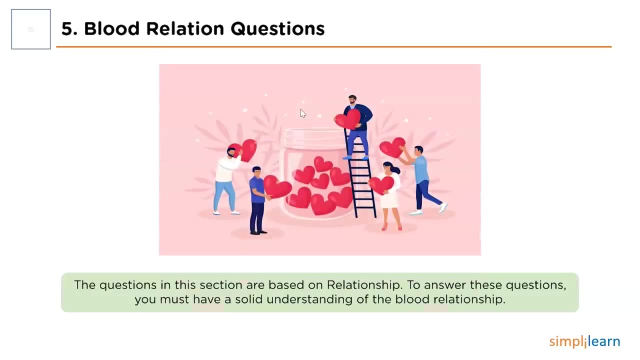 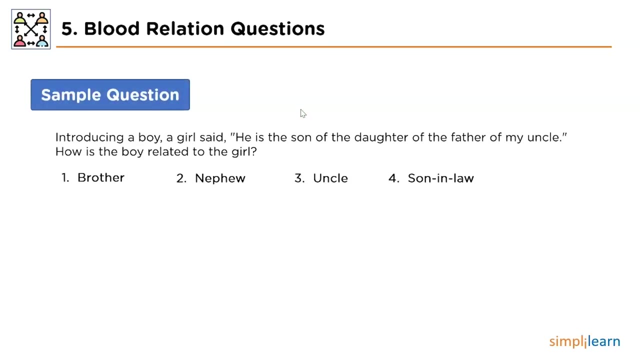 The next topic is blood relations. The questions which are asked in this section depend upon relation, So you should have a sound knowledge of blood relations in order to solve these questions. Let's look at one sample question to get an idea about how these blood relationship questions work. 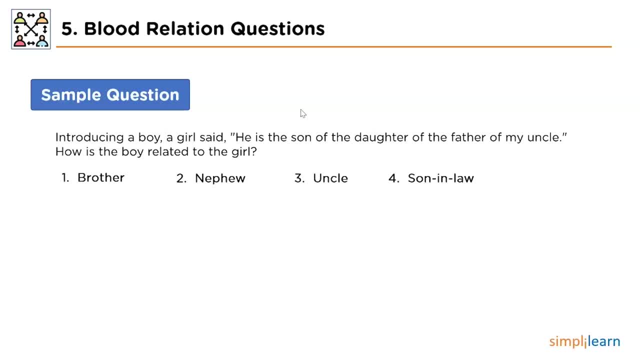 The problem statement given here states that, Introducing to a boy, a girl said He is the son of the daughter of the father of my uncle. How is the boy related to that girl? Let's figure out an answer to this question by breaking the problem statement into chunks. 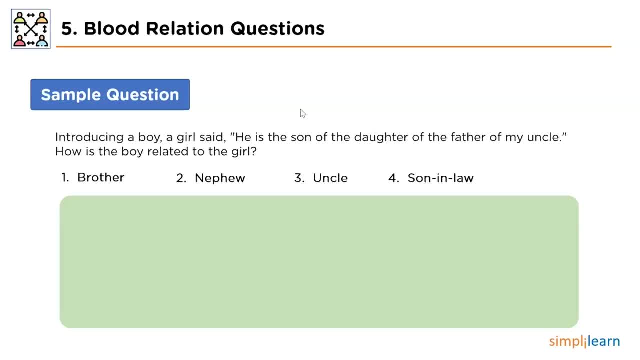 We'll start tracing the problem statement from backward direction. The highlighted part says father of my uncle And uncle's father is nothing but the grandfather. This grandfather has a daughter, So we'll add that daughter here, And this daughter has a son, whom this girl is referring to now. 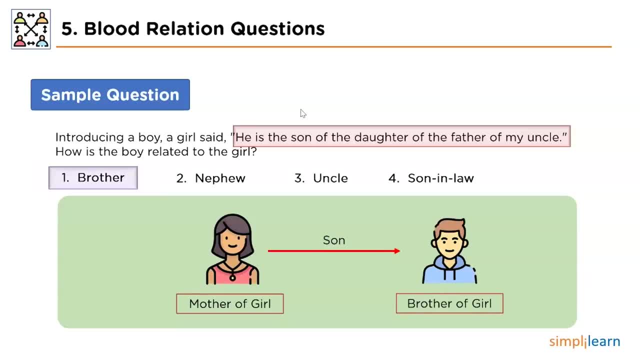 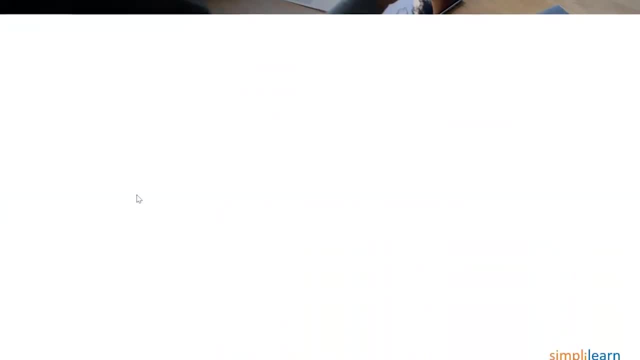 This means The guy in the picture is girl's brother, which is option 1.. The next topic is clock. The questions in this section are based on time and clocks. You'll come across questions such as measurement of angles between hands of clock. 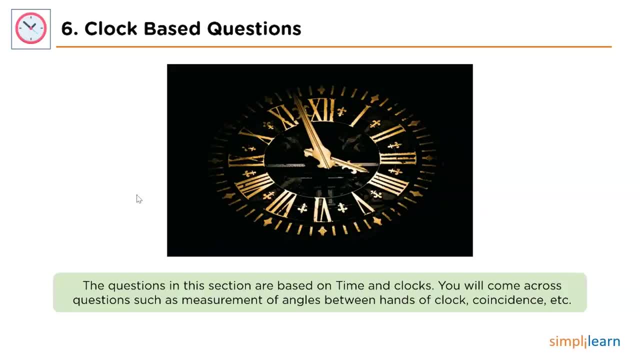 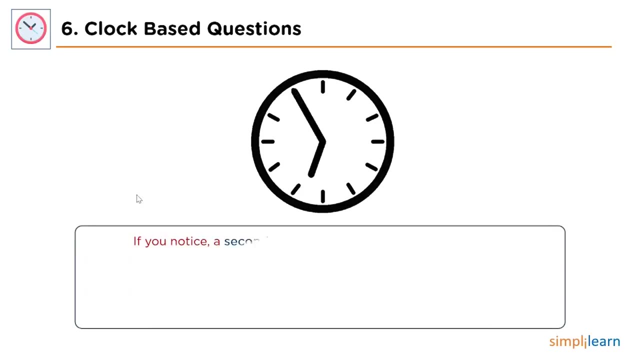 coincidence between hands of clock, time, when particular angle between hands of clock is given, time lost in a false watch, etc. Let's understand the concept of clock first. In a watch, a second hand covers 360 degrees within 60 seconds. 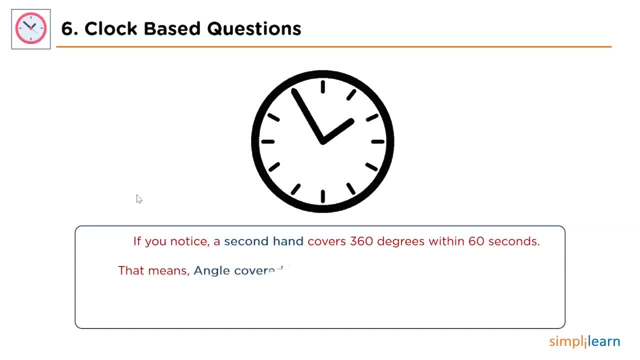 How much angles do you think a minute hand will cover? Well, a minute is nothing but 60 seconds. So if we divide the measurement of a complete clock by 60, then we should get the angle covered by a minute hand. And 360 by 60 is nothing but 6 degrees. 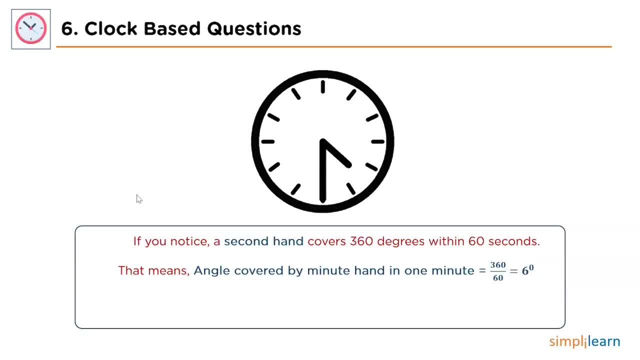 So 6 degrees will be the angle covered by minute hand in 1 minute. Similarly, if you compute angle covered by hour hand in 1 minute, that is 360 divided by 12 hours into the conversion of an hour into minute. 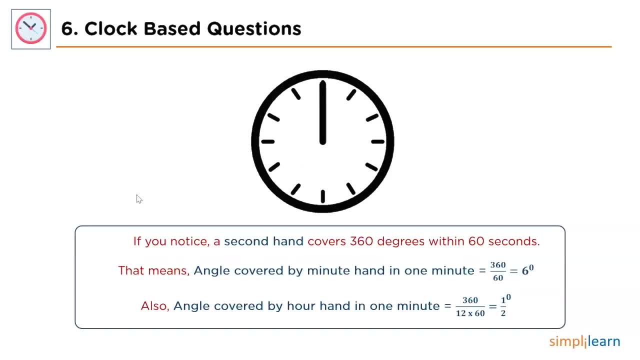 that is 60,, which will further result into 1 by 2.. Now we know that both the minute hand and hour hand will move in same direction, that is in a clockwise direction. Hence we can also compute the relative angular displacement. 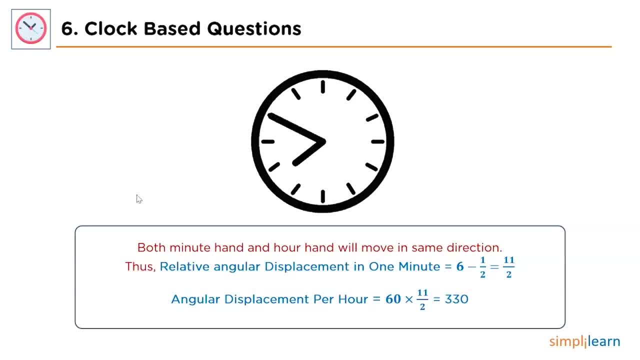 which will be nothing but the comparison of difference between the angular displacement of both these hands of clock per minute. So, doing that, which is 6 minus 1 by 2,, we will get 11 by 2 as an answer. This is angular displacement per minute. 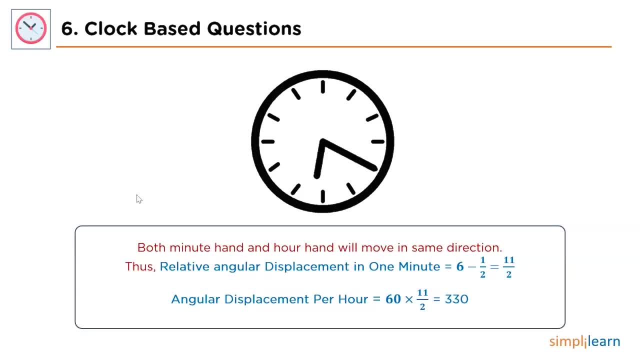 Now, if we multiply this value by 60, we will get an angular displacement per hour which is 330 degrees. Also, any angle more than 180 degrees is called as reflex angles, And in solving clock questions, we always try to refrain from reflex angles. 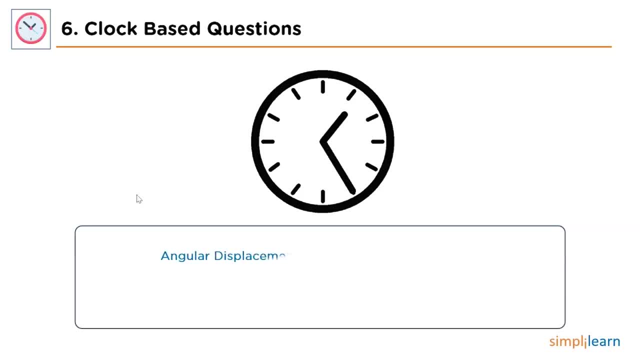 So we will convert this angle into non-reflex angles. To do that, all you have to do is subtract the value from 360.. Doing that, we will get 30 degrees as our non-reflex angle value. Moving ahead by using formulas we derived by angular displacement per hour and per minute. 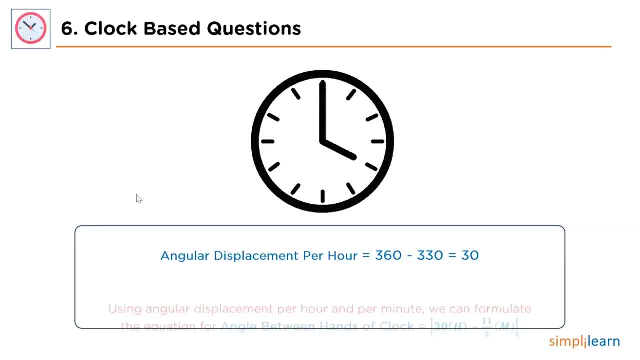 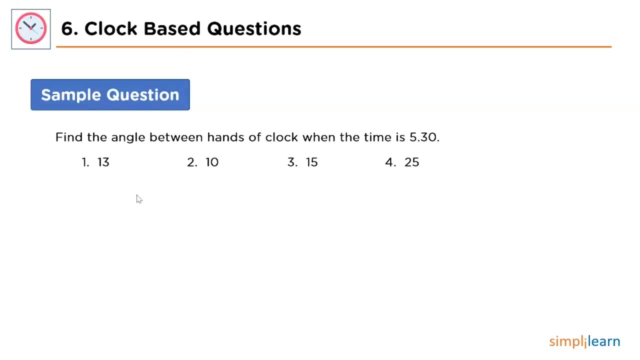 we can formulate the formula for an angle between hands of a clock and that will be mod of 30h minus 11 by 2m. h here is our value and m here is nothing but minute value. Let's look into a sample problem to comprehend the application of this formula. 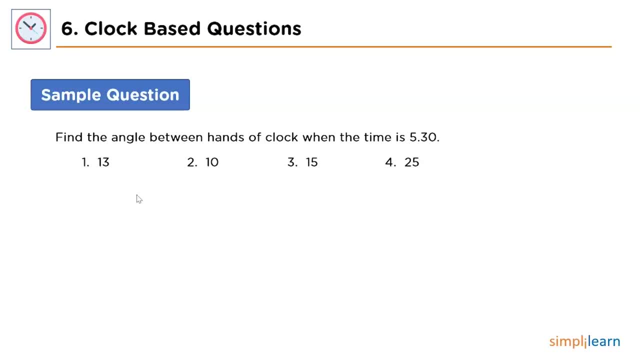 The problem statement asks us to evaluate the angle between hands of clock when the time is 5.30.. The answer to this question is pretty straightforward. All you have to do is the fill value in equation. The edge value is 5 in this case and m value is 30.. 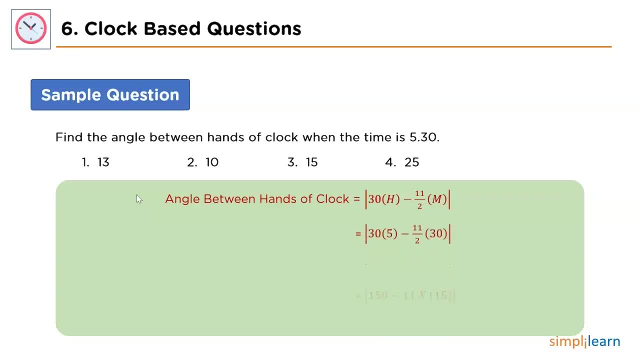 Now, 30 into 5 will be 150, and 11 by 2 into 30 will be 11 by 15.. After further computation will get 15 as an answer. We will look at one more type of clock question. 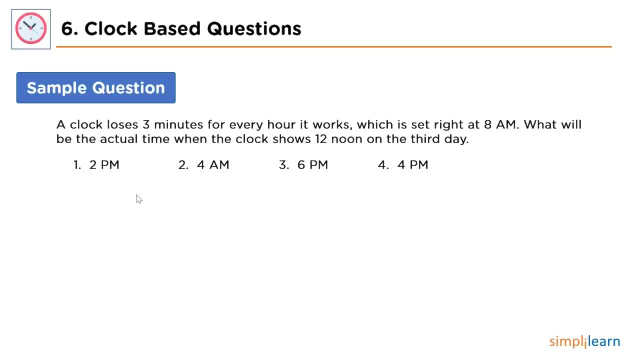 The question given here says that a clock loses 3 minutes for every hour it works, Which is set at right 8 am. What will be the actual time when the clock shows 12 noon on the third day? Let's look at this problem statement closely. 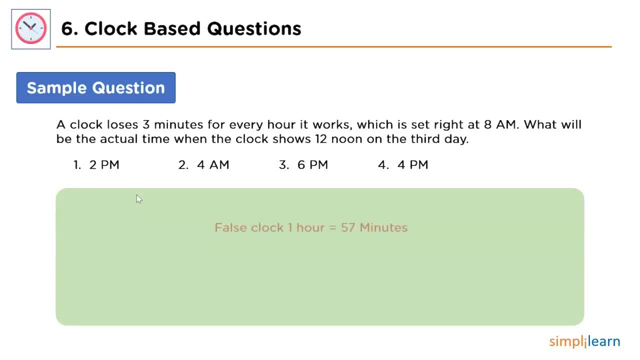 It says that a clock loses 3 minutes every hour. That means 1 hour is equal to 57 minutes. Also, this Paul's clock started at 8 am and stopped at 12 noon after 3 days. So the number of hours completed by a Paul's clock is 24 into 3, that is 30.. 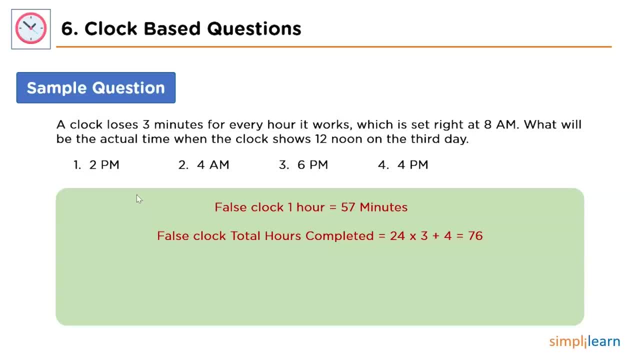 Plus extra 4 hours between 8 am to 12 noon, which equals to 76 hours overall. Now we want to find out the hours covered by true clock in order to predict the accurate time, And we know that our first clock has covered 76 hours, where each hour equal to 57 minutes. 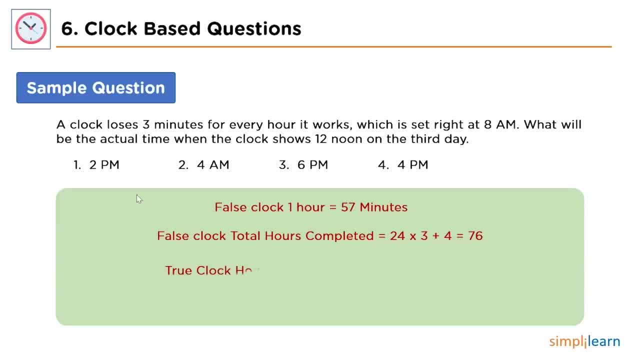 From this we can say that the true time will be 76 into 60 divided by 57.. This equation will give us the right hours covered by the clock, which is 80 hours, And since the time covered by the true clock is 80 hours, we will have to add an extra 4 hours time to 12 am. 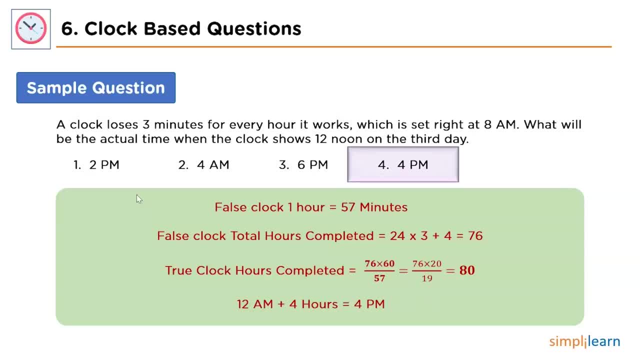 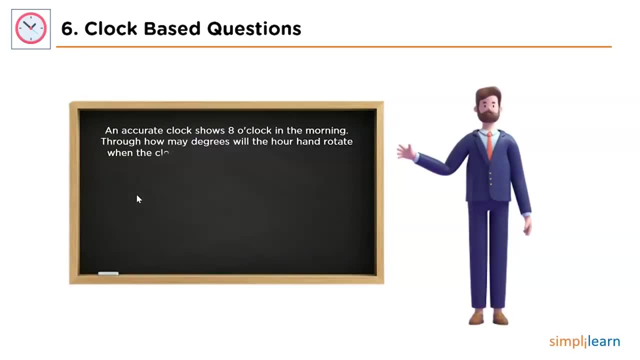 Hence our answer will be 4 pm. On that note, here is a sample question to check your understanding of clock concept. All of you guys can solve this question and drop your answers in the comment box below. To do that, I will provide you with a short moment. 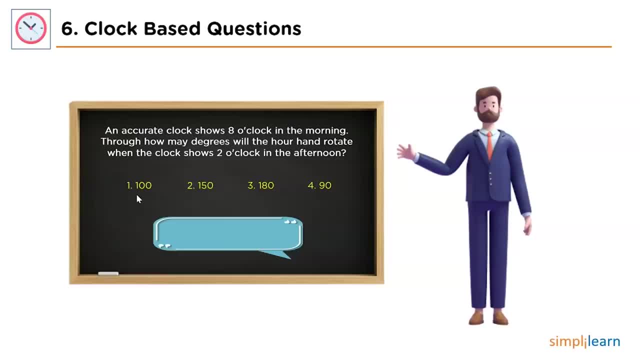 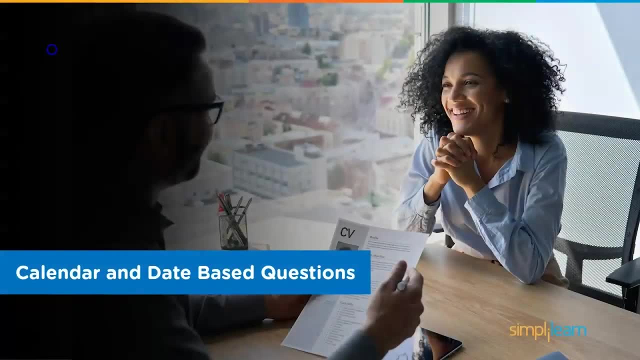 I hope that all of you guys have solved this question and dropped your answers in the comment box below by now. Moving forward, we will discuss the section of calendar and date based questions. The questions in this section will test your understanding of the calendar concepts. 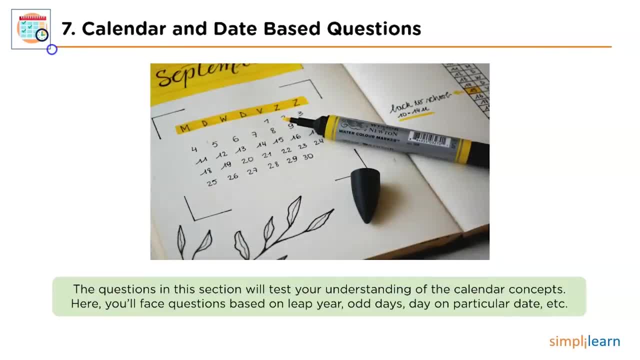 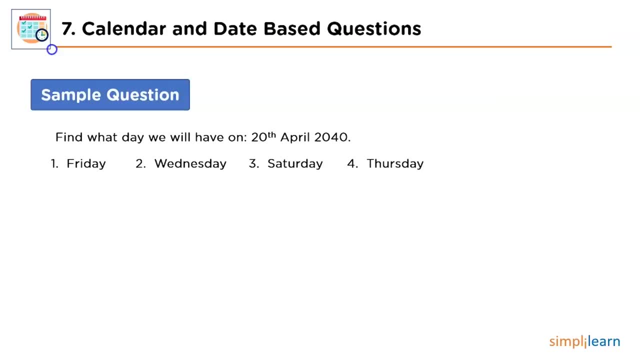 Here we will face questions based on leap year, odd days, a day on a particular date, etc. Let's look at a sample question to figure out how questions in this section can be print. The problem statement given here is asking us to find out what day there will be on the date 20th April 2015.. 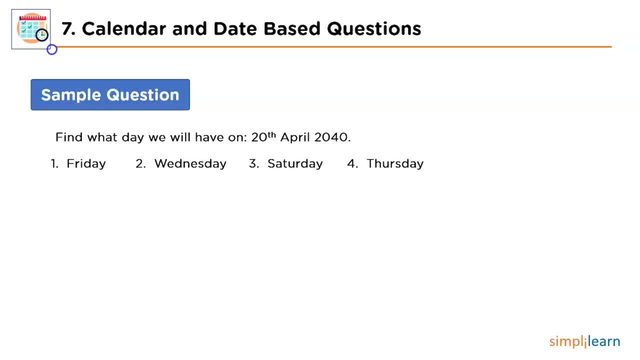 Now let me tell you, we can figure out an answer to this question within 30 seconds by using a really interesting trick. This trick begins by breaking down the given data into 5 sections. For home, we will compute odd days, which will finally lead us towards the day evaluation. 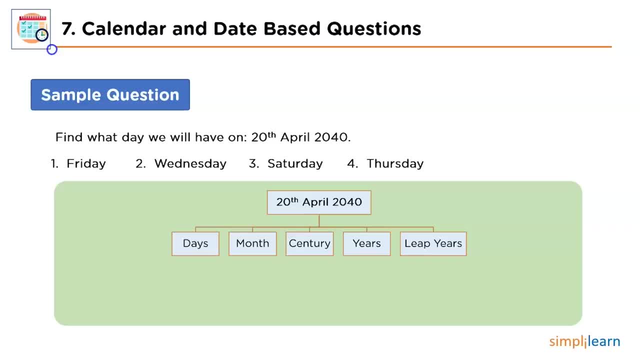 And those 5 sections are days, months, century, ordinary year and leap year. Let's understand how we can figure out the answer using this data. So we have a date value as 20.. Then we have month as April, Then we have century as 2000.. 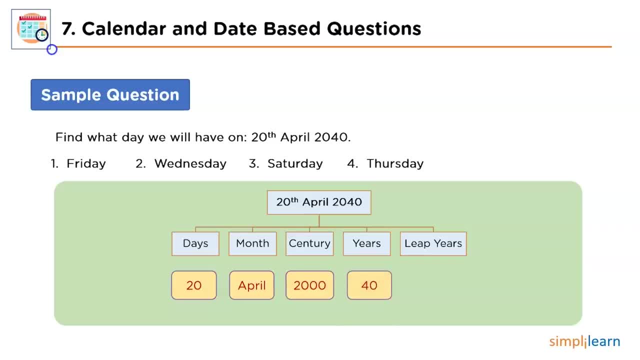 And ordinary year is 40. And leap year? Now, what is a leap year? Well, you must know that leap year occurs after cycle of 4 years, And if we divide the ordinary year value by 4, then we should get the leap year value, which is 40 by 4 and 10.. 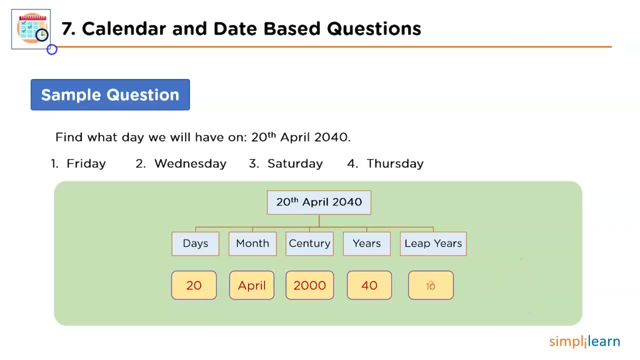 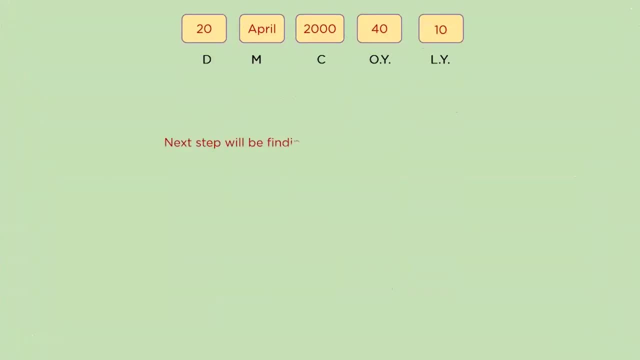 In this case. Now we will move towards the next step, which is nothing but the odd day calculation. First we will figure out odd days for the date section. In a week we usually have 7 days. Thus odd days can be considered as the remainder of number of days by week days. 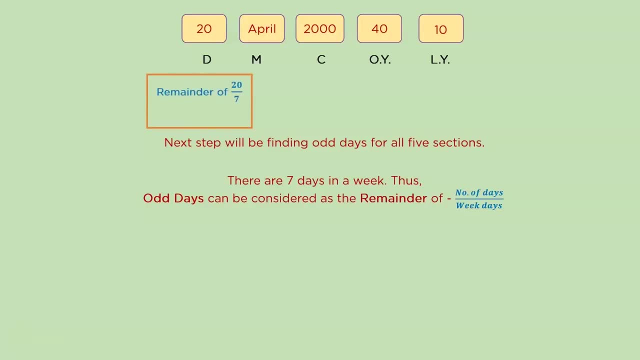 Which will be the remainder of 20 by 7 in our case, And that is 6.. For next two factors, that is, month and century, we have predefined odd day values. So, moving forward, we will discover them. These are the odd day values for month. 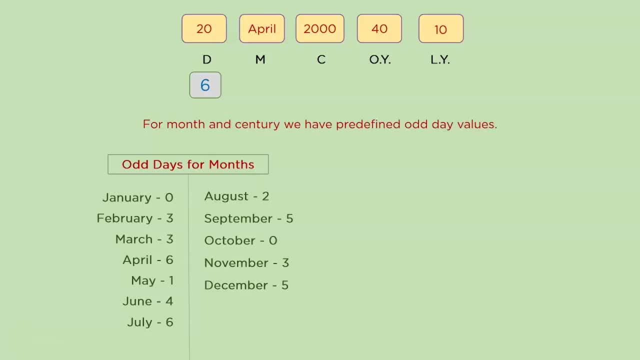 You will have to remember these values to be able to answer these type of questions using this trick. Let's also look into the odd day values. for centuries, These values work the same in forward direction as well as the backward direction. What this means is, for century 2100 to 2199,, you will again have odd day value as 4.. 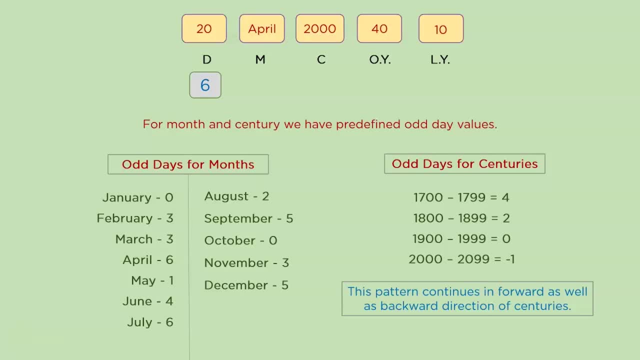 For 2200 to 2299, you will have an odd day value equal to 2.. I hope this is clear to all of you guys. From these tables we can add the odd day values for our month and century section. For month, we have odd day value as 6.. 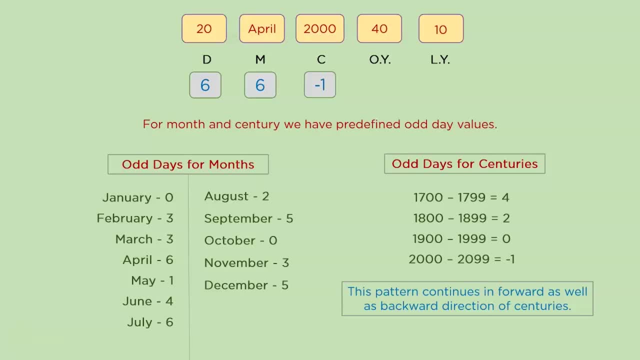 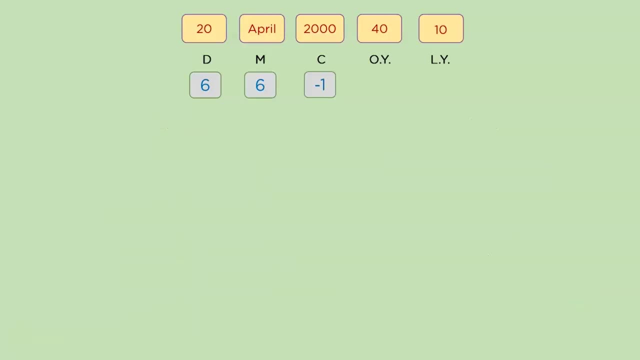 Odd day value as 6.. And for century we have odd day value as minus 1.. Now the only part left is ordinary year and leap year. And if you remember, in an ordinary year we have only one odd day. 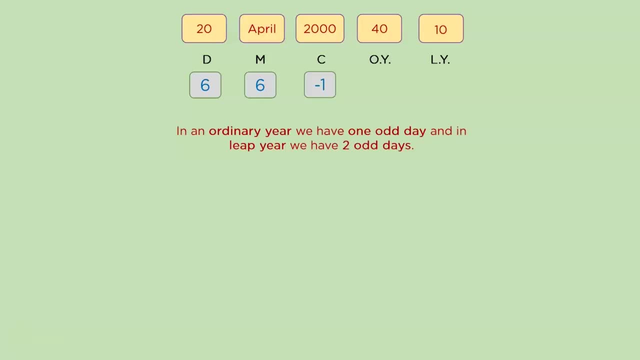 And in a leap year we always have two odd days. So according to this logic, we will add 40 odd days for ordinary year, And we have covered leap years inside these ordinary years as well. So we will add only 10 odd days for leap year section.